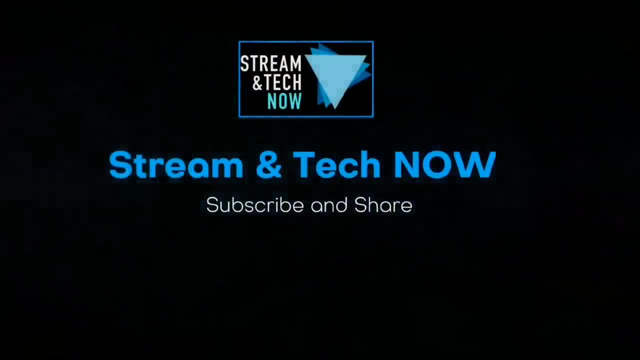 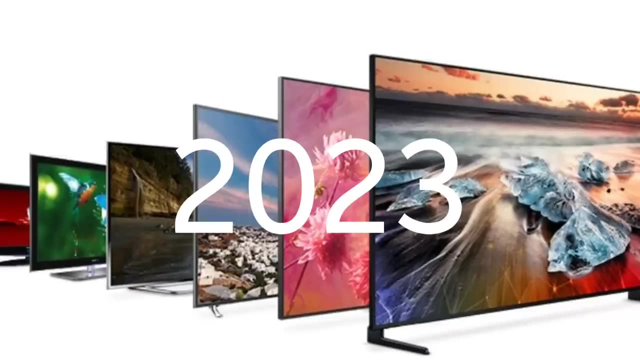 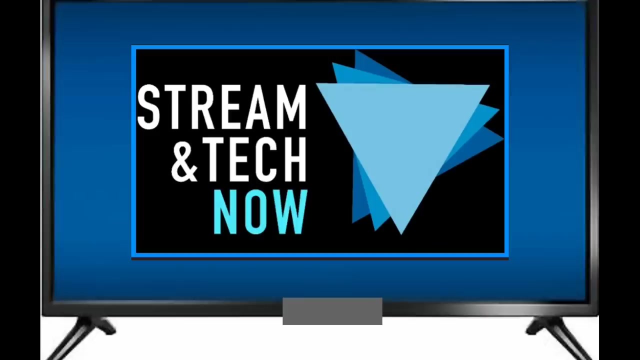 coming up next. Now I'm going to go from worst to best. Now. this is the latest 2023 result, Based on a multitude of factors. some of the most popular brands will be discussed, and make sure you stick around for the very end, as I will reveal the one brand you need to stay far away from Now. 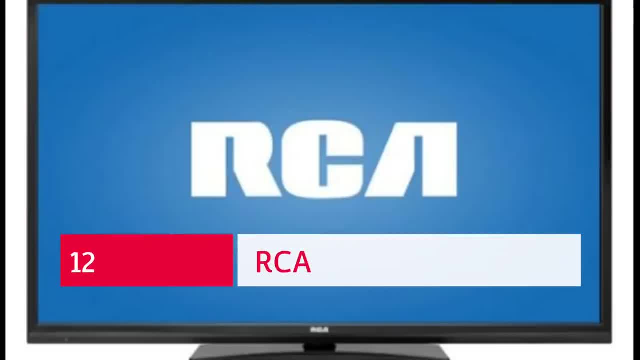 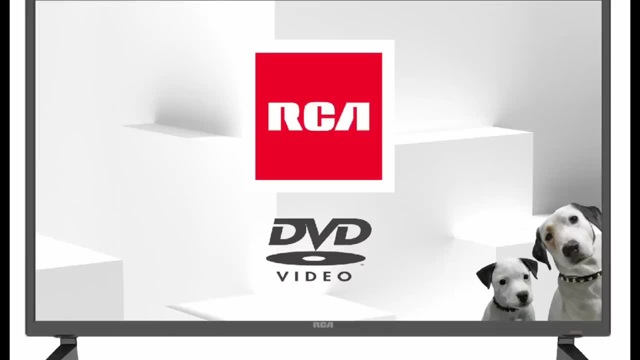 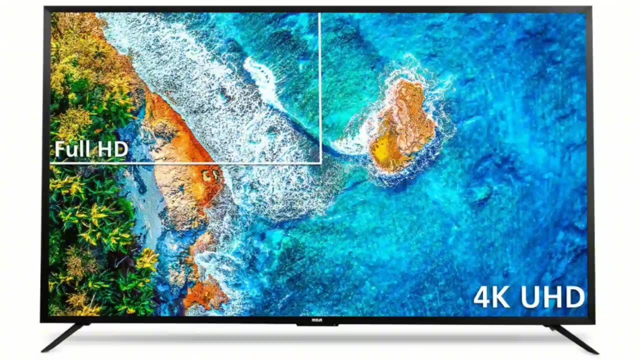 coming in at number 12 is RCA. Despite being one of the oldest electronic brands in American history, RCA's continued decline amongst its peers makes it one brand to avoid. Now, RCA televisions are typically between 30 inches and 50 inches. They've been criticized by consumers due to inconsistent. 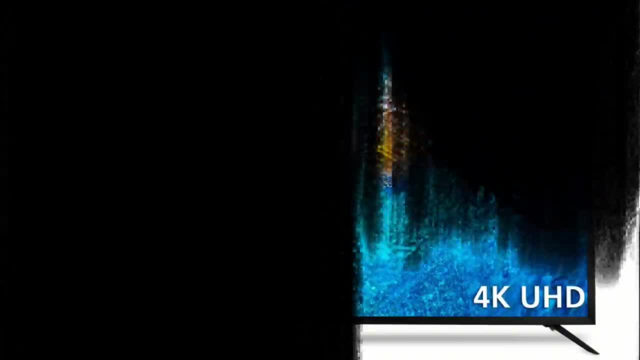 picture quality. They've been criticized by consumers due to inconsistent picture quality. They've been criticized by consumers due to inconsistent picture quality. Narrow angle of view, The negative consumer feedback, make this brand one to avoid. Number 11, Insignia: Now, this is the 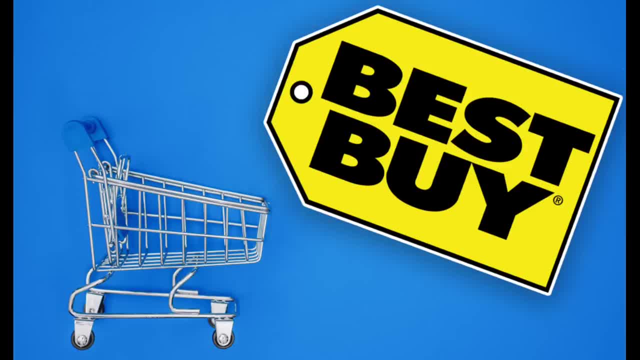 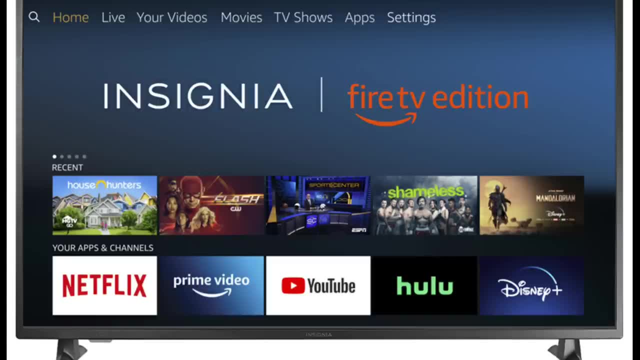 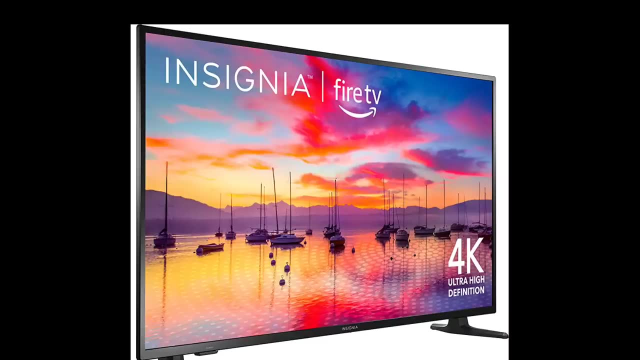 best by electronics brand. It makes one of the best selling budget televisions on the market. Most Insignia's cost under $500.. Now this brand falls short of quality when you put it against its competitors from a technical standpoint. Now Insignia televisions also lack the same level of. 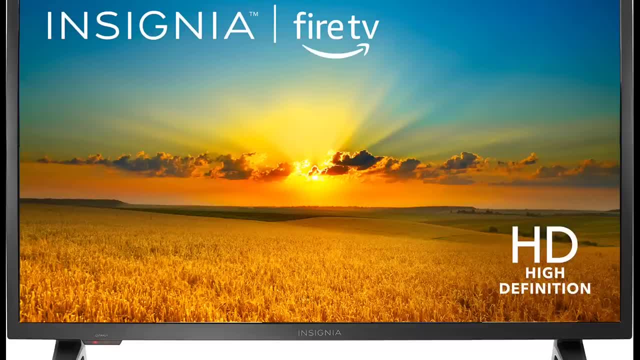 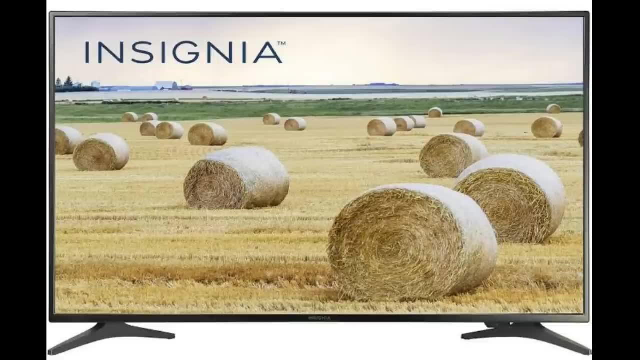 HDR support as its competitors. It maxes out at about a hundred percent of its competitors At HDR 10,. Insignia products also lack local dimming, opting for a more cost-effective but worse looking direct lighting. As a result, these televisions lack the contrast and highest peak. 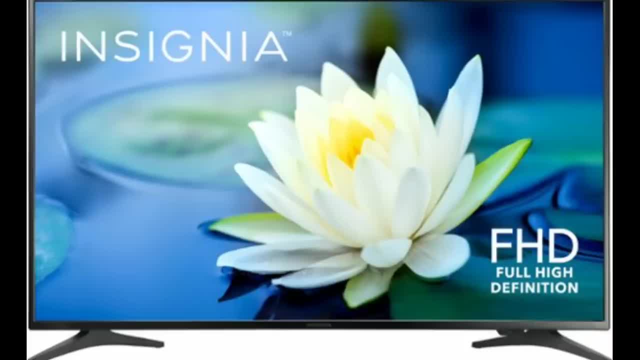 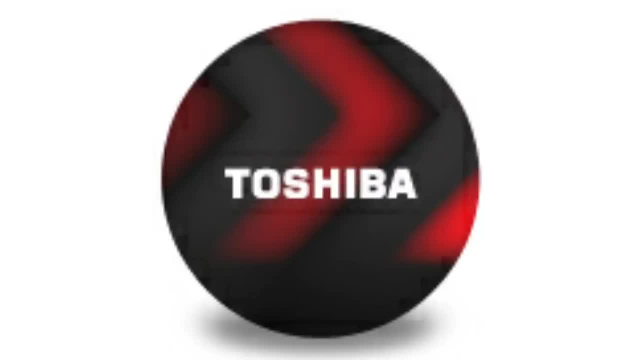 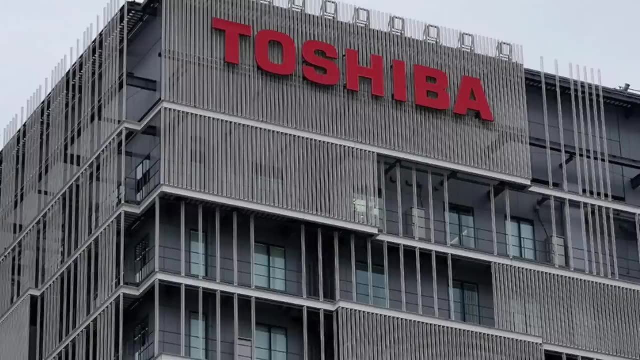 brightness of other televisions in its comparable price range, Coming in at number 10, Toshiba. Now, Toshiba's reputation in the television business is not what it used to be and has been purchased by Chinese manufacturer Hisense. However, Toshiba continues to operate as a separate. 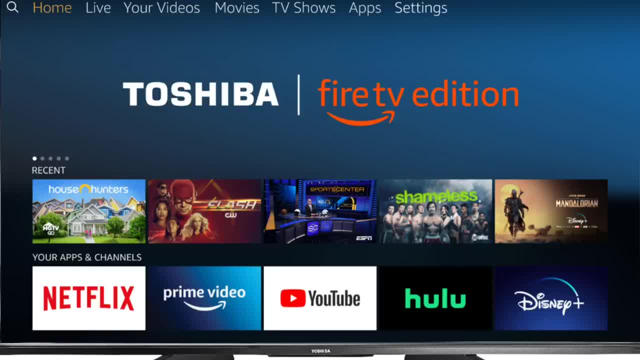 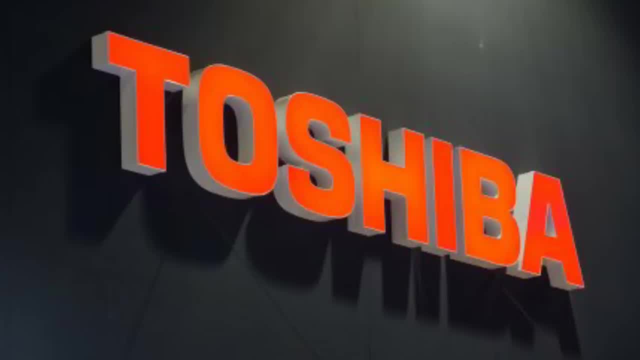 entity and may be the optimal television for those seeking the familiar look and feel of the Amazon Fire TV operating system. Now, Toshiba televisions have a lower latency time when used in conjunction with modern consoles. Toshiba also has a slight edge in its port selection. 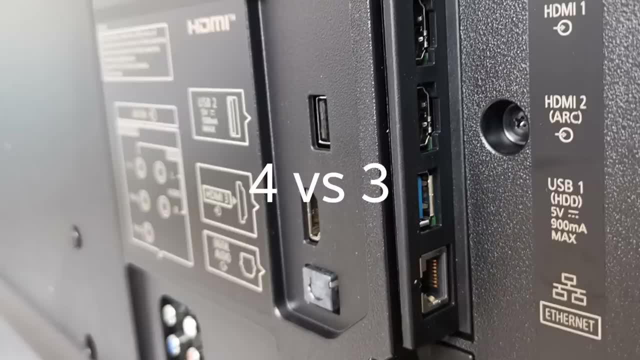 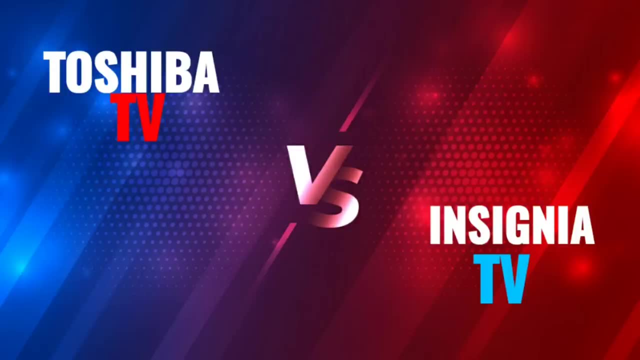 offering four HDMI ports to Insignia's three, And, as a result, Toshiba's televisions continue to have a leg up on Best Buy's Insignia brand. In spite of their overwhelming similarity, they do fall short of other companies that produce a better product. 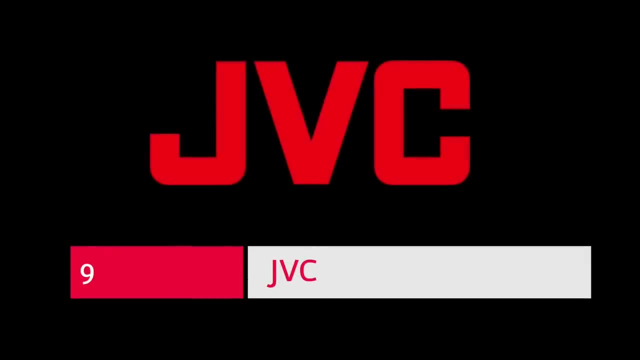 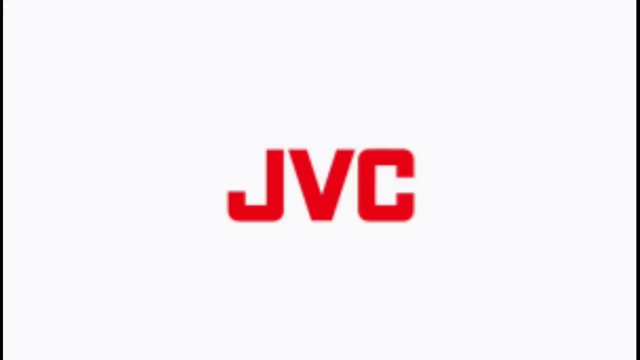 Number nine: JVC. While JVC is a respected and reputable brand in global electronics, the Japanese company isn't one of the top major television brands in the world. It lacks the market share and sales volume of its competitors. Nonetheless, they have cultivated a loyal customer. 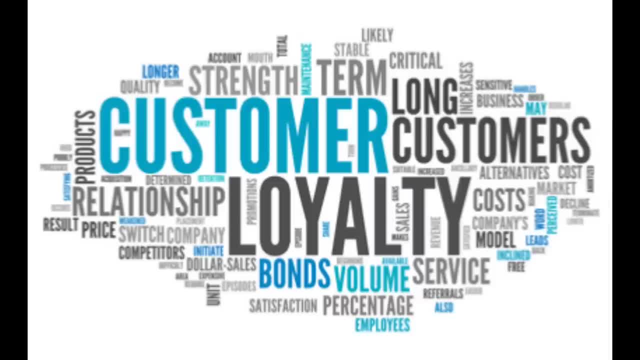 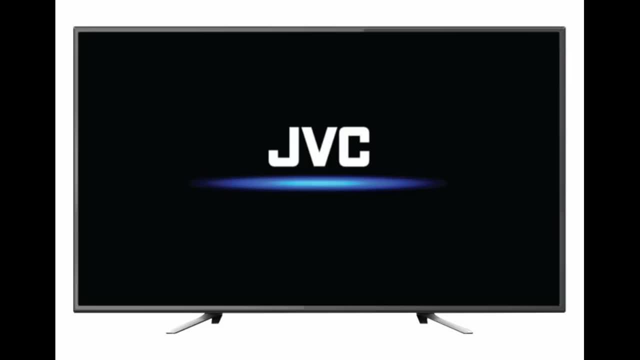 base over the years. Now, one of the brand's drawbacks includes its inconsistency in worldwide distribution. JVC televisions are just not readily available to the public, So Toshiba's available in the United States as they are in other countries like Australia, etc. Therefore, 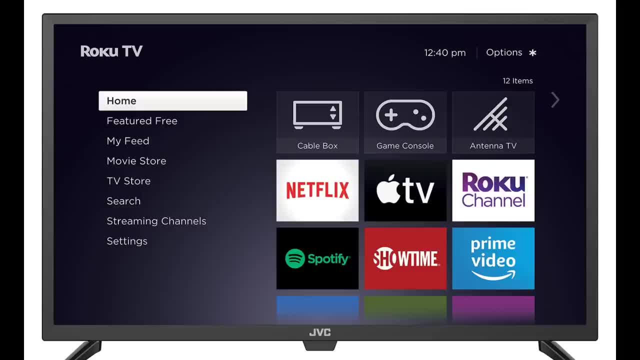 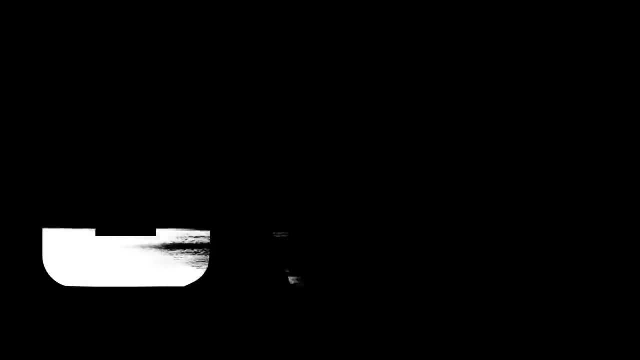 the choice of models could be limited. for US consumers, There is also an inconsistency in the operating systems they use. They utilize one of several operating systems for its televisions, depending on what region of the world they are made for, So the technical specs can cause it. 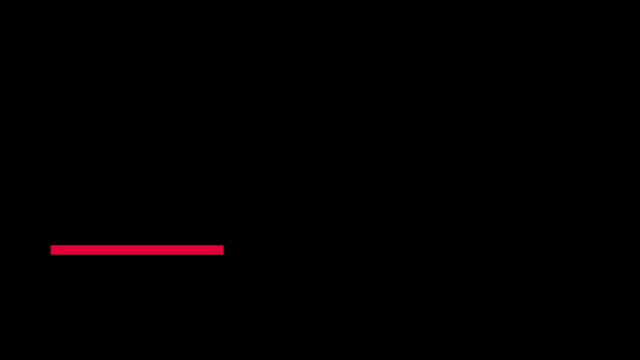 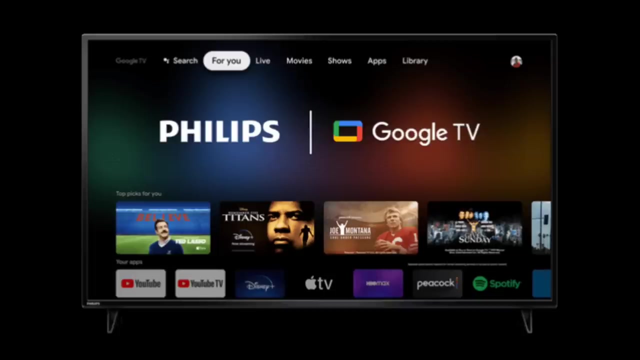 to fall short of their overseas competitors. Coming in at number eight, Philips, Now similar to JVC. Philips is not accessible in all parts of the world. Now, Philips is not accessible in all parts of the world, The Dutch company, despite having origins dating all the way back to the 19th century. 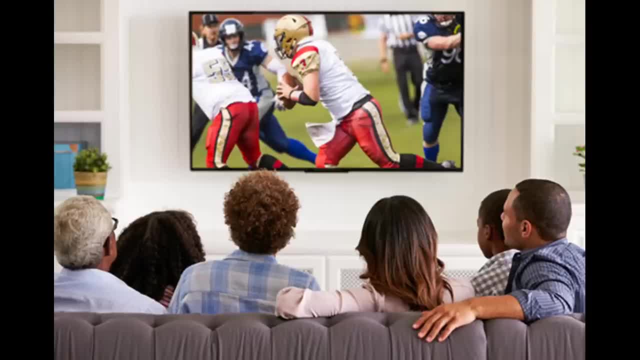 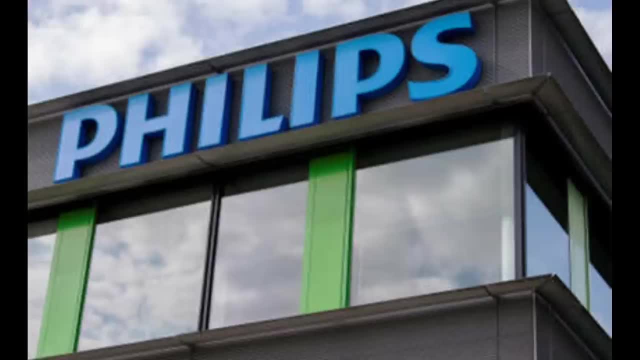 does not currently manufacture televisions for the American audience. Instead, they sort of focus on the European and the Asian markets And as a result, it falls behind some of the mainstream competitors. However, Philips is still known to produce a quality product for its consumer base. 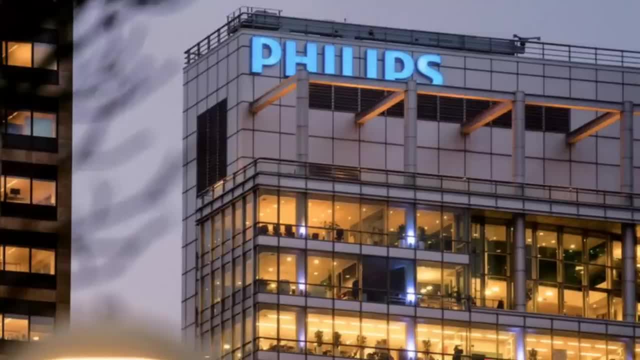 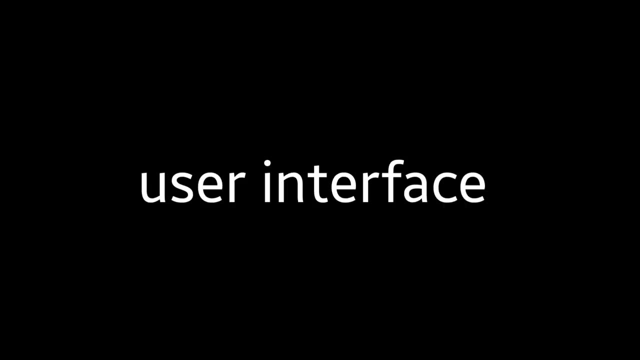 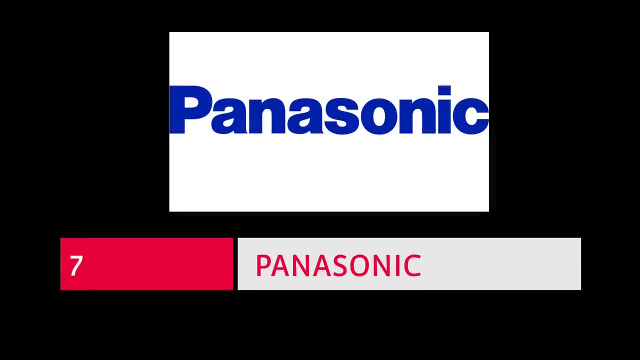 offering a full array of display technologies, But the Dutch company is not without its drawbacks. There are lots of complaints of the user interface and how it lags behind other systems. Buyers have frequently reported problems with stuttering and buffering within the menus. Number seven: Panasonic Now since 2016,. Panasonic televisions are quite limited in North America. 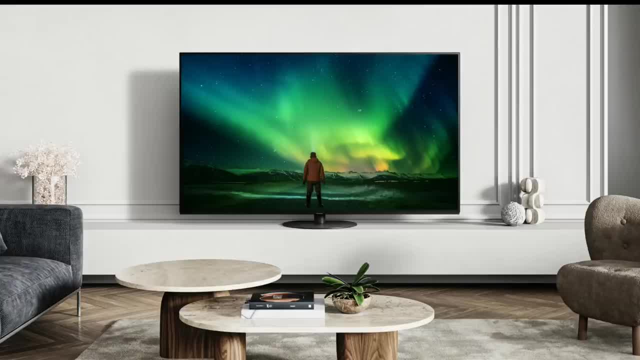 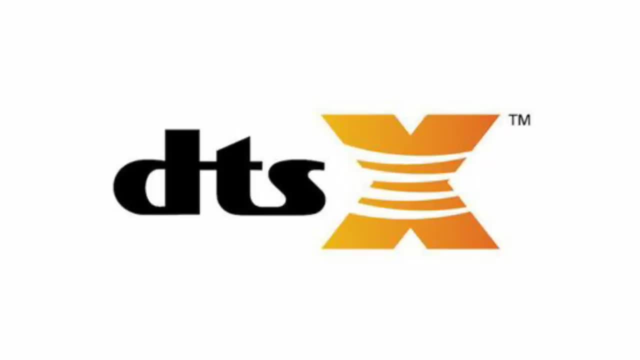 Most Panasonic models are known for their durability and sustainability. They do seem to offer advanced audio technology such as Dolby Atmos and DTS-X that lend to a higher quality sound than most of its competitors. However, the brand still has its drawbacks, such as limited 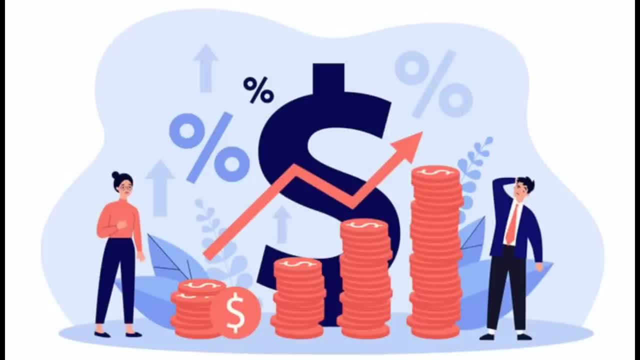 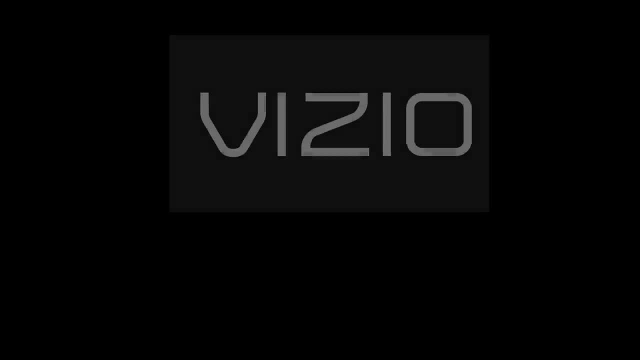 selection in its app store compared to its competitors, as well as its pretty high price point. Number six: Vizio. Now, this company offers a better picture quality than some of the world's most popular budget brands. While Vizio may be the preferred budget television brand to many, 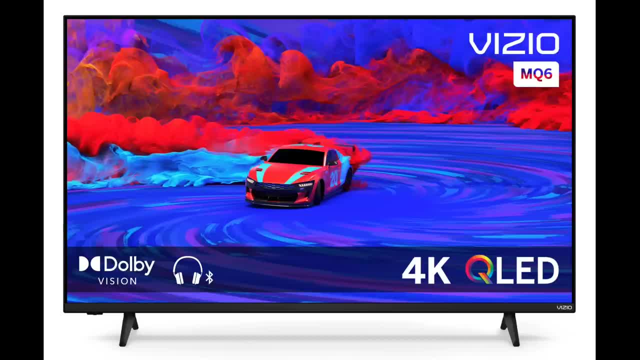 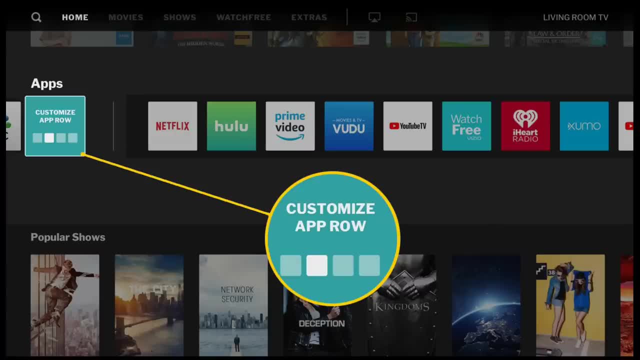 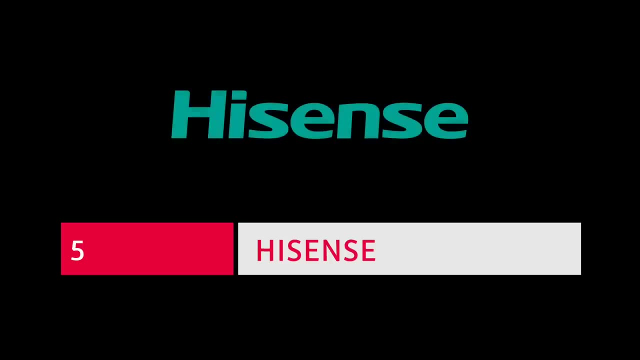 the company's televisions are by no means perfect. Some consumers have reported issues with build quality and durability. They also suffer from a similar problem to brands like Panasonic, such as a lack of a quality app selection and a clunky user interface. Number five: Hisense Now. Hisense has been around for more than 50 years and it's the largest TV. 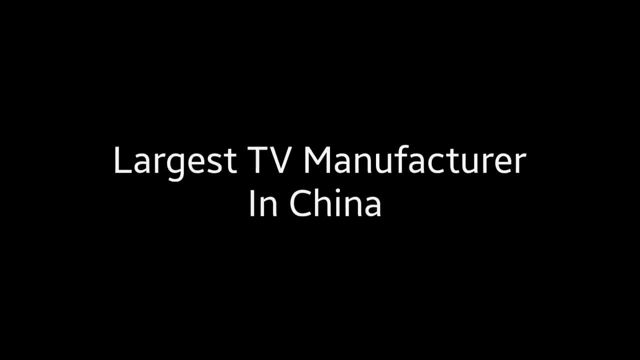 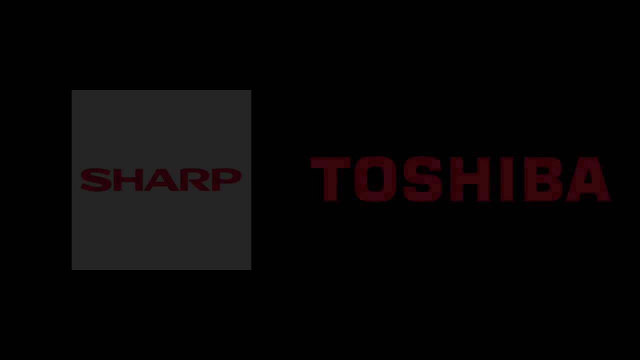 manufacturer in China. The company has seen further growth by investing in name legacy brands such as Sharp and Toshiba. Now a few of Hisense's complaints, and one of its biggest drawbacks is its audio quality. They also have negative feedback for being flimsy and have a brittle. 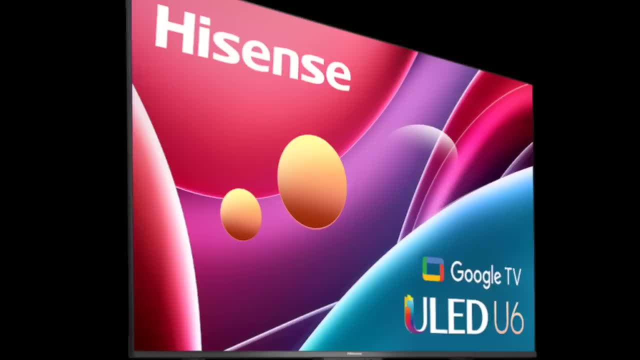 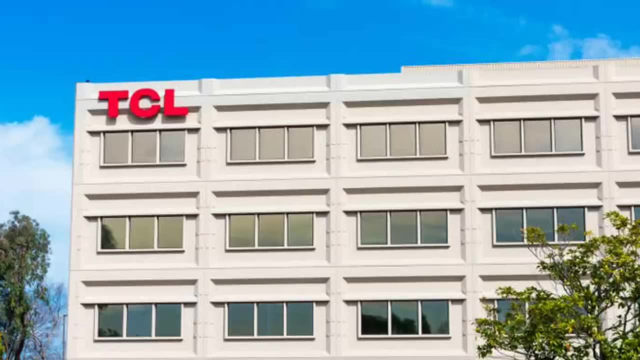 design, but it definitely offers a viable option for some of its higher price competitors. Number five: Toshiba. Now Hisense has been around for more than 50 years and it's the largest TV. They've become one of the fastest growing brands in the world. However, customer frustrations with 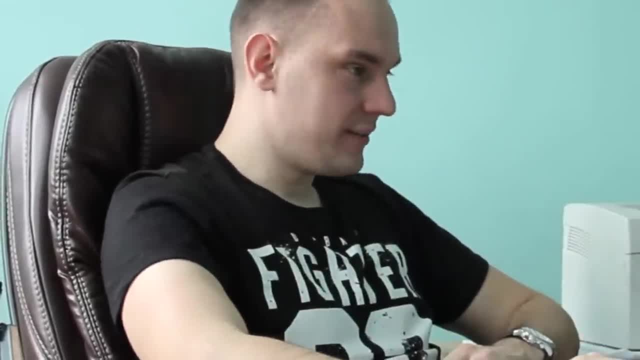 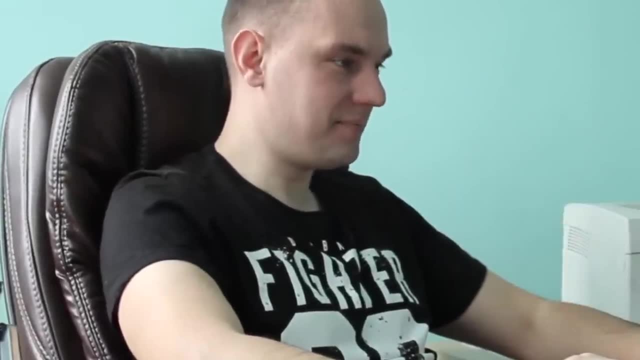 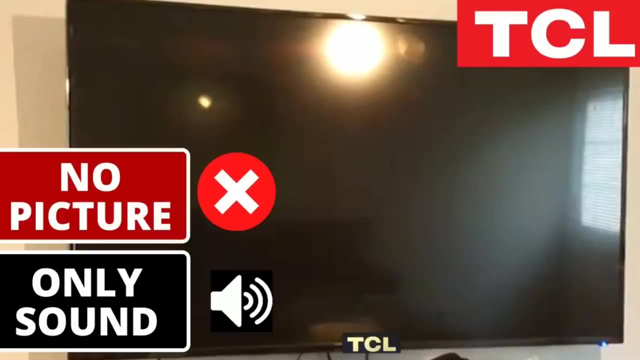 customer support, in addition to inconsistency with the out-of-box product, prevents TCL from entering the top three. A lack of quality control over the final product has seen several consumer reports: dead pixels on the screen. Additionally, some models make use of cheaper materials that 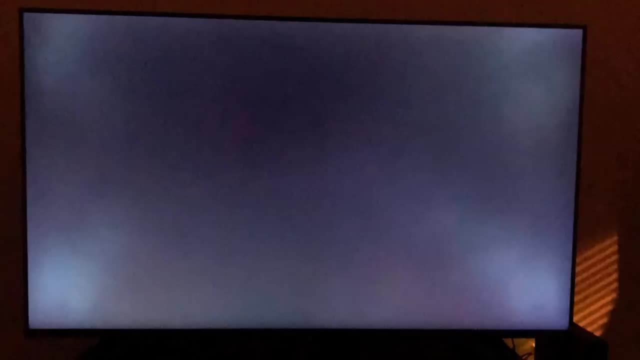 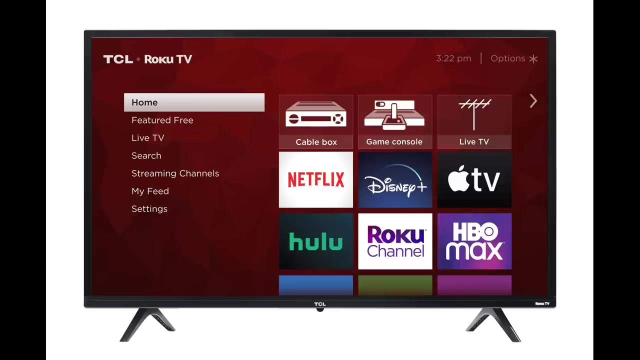 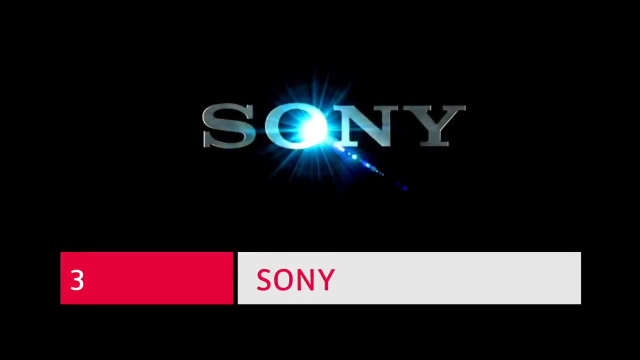 can result in screen bleeding and other defects. However, TCL's use of familiar operating systems such as Roku and Android should mitigate these problems for users looking for an easy-to-use and easily navigable user interface. Number three: Sony. Now, Sony has managed to maintain a hold. 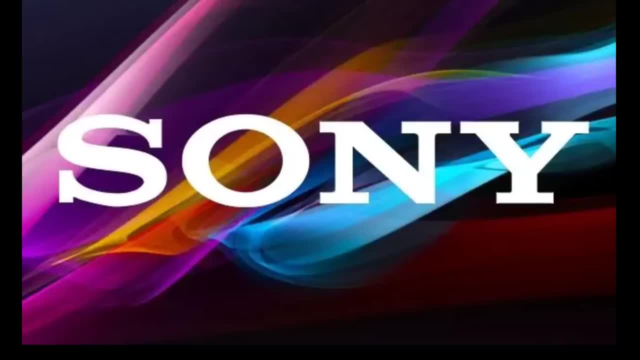 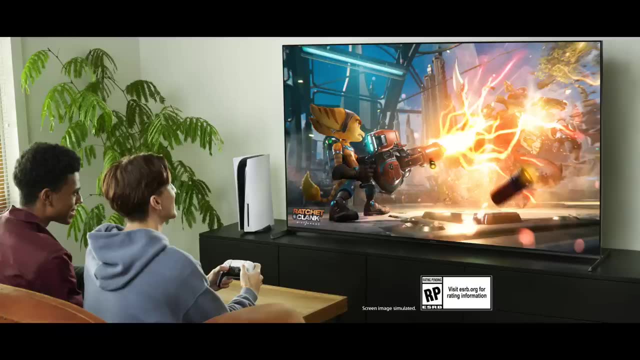 on the television market, specifically thanks to its high picture quality. With all the modern innovations packed into sleek and modern designs, Sony devices make for great gaming televisions and also utilize a built-in feature known as Sony Music. While consumers are sure to receive a strong product, out-of-the-box, with dedicated audio. Sony has also managed to maintain a hold on the TCL market, specifically thanks to its high picture quality. With all the modern innovations packed into sleek and modern designs, Sony devices make for great gaming televisions and also utilize a built-in feature. 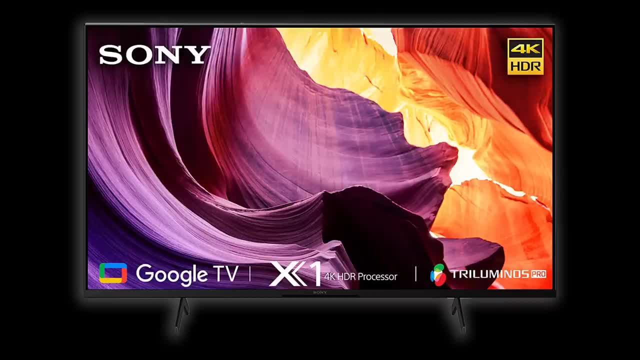 that makes it easy to maintain a hold on the TCL market, specifically thanks to its high picture quality. While consumers are sure to receive a strong product out-of-the-box with dedicated audio, there are cheaper options. Sony televisions also lack security backups, like some of its 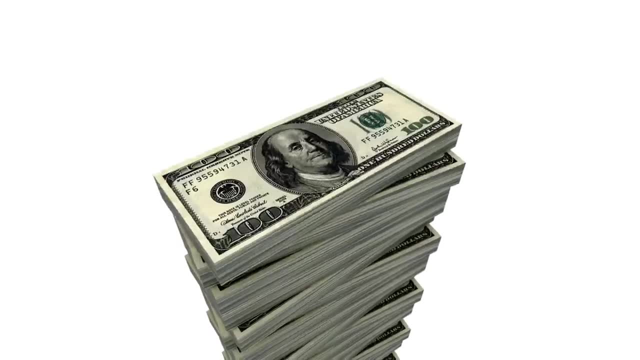 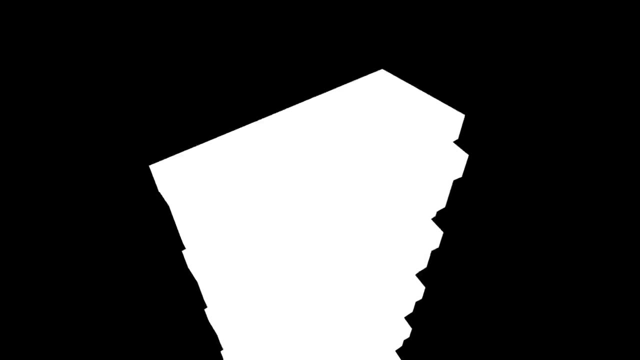 competitors, Though the biggest obstacle standing in the way of consumers bringing a Sony television home to their living room is price, as most higher-end models cost upwards of $2,000.. The final two: if you see some list, they might be flip-flop Nonetheless. 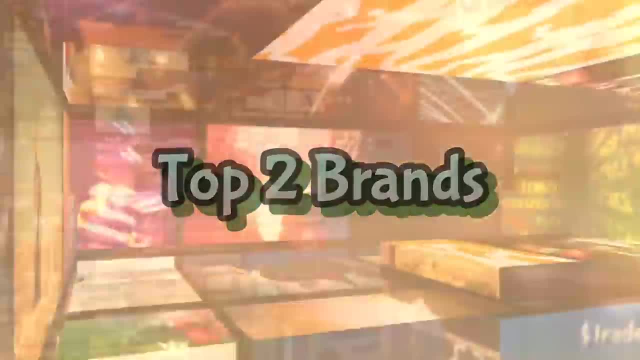 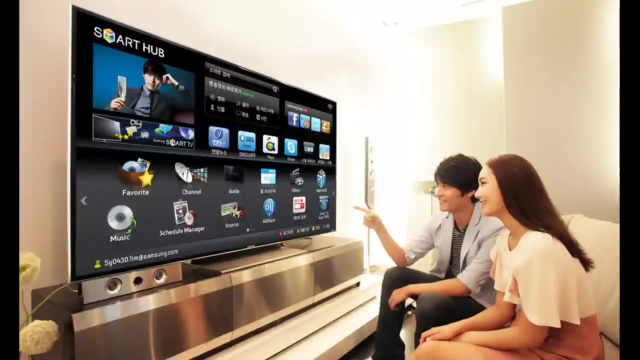 these are the two top brands when it comes to televisions. Coming in at the number two spot is Samsung. In addition to its premium price point, Samsung is also a great brand for its TVs. Samsung TVs also display an abundance of ads that can be a nuisance for consumers. 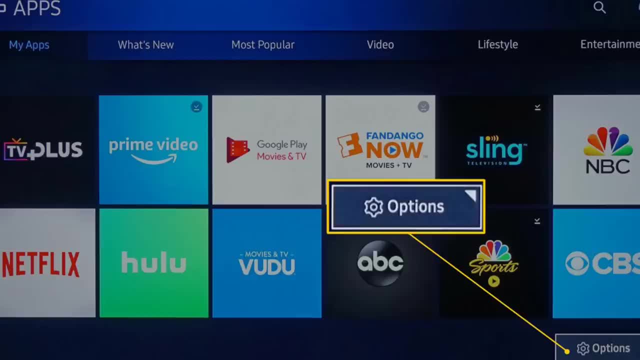 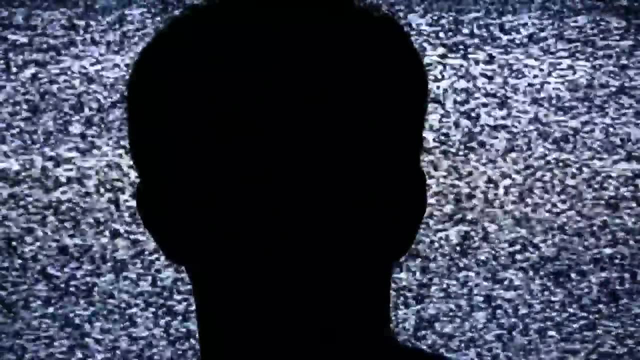 Additionally, some Samsung televisions may come with an abundance of bloatware or pre-installed apps that may not be necessary for an optimal experience, But if users can get comfortable with these items, they can rest easy knowing that they are getting one of the most. 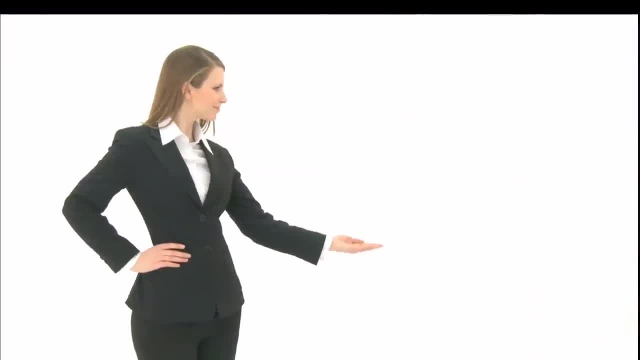 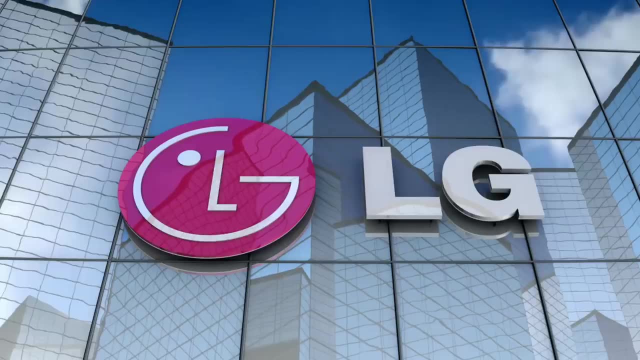 premium televisions on the market. Finally, the number one spot has to go to LG. Looking for the highest quality television on the market should look no further than LG, The South Korean company. Samsung is one of the most popular televisions on the market. The number one spot. 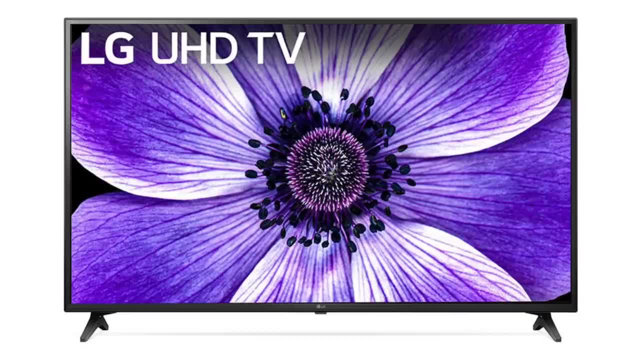 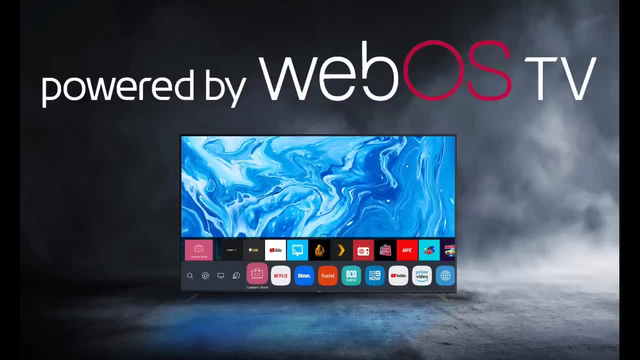 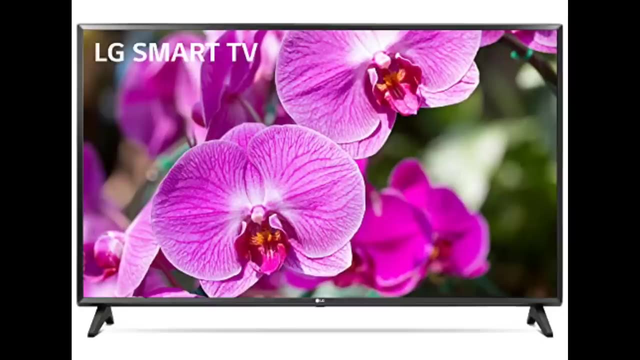 has built a reputation for durable and aesthetically pleasing designs on all models. They also get quite a bit of positive feedback on their webOS smart TV software, with reviews indicating a smooth and easy-to-use operating system among all major television brands. Personally, though, I think that is quite subjective, as it's not one of my favorites. 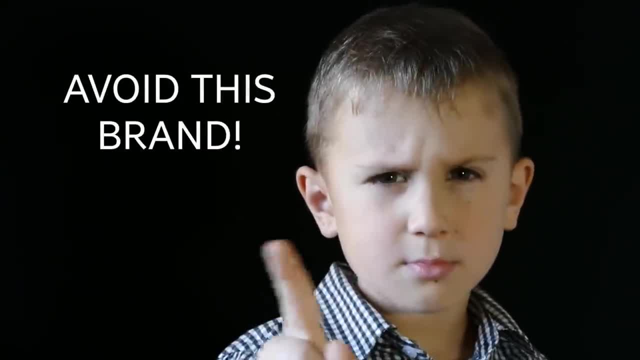 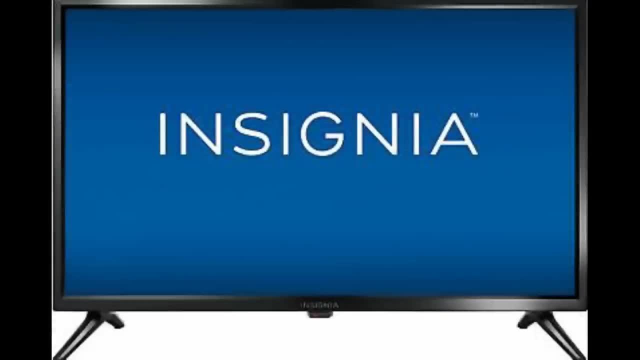 Earlier in the video, I promised to tell you the brand to stay away from, so here it is. In my opinion, you should stay far away from Insignia, which, in all honesty, is due to my personal experience, as well as family and friends also sharing similar experiences with this brand. 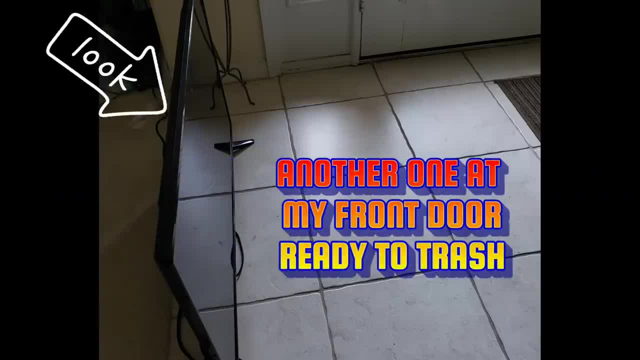 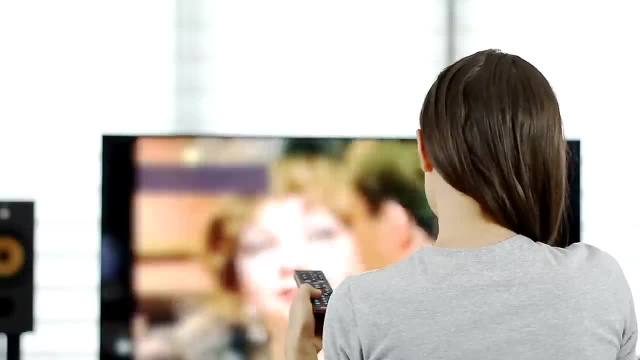 Now I've had three and every single one of them has not lasted long. It just completely stops working, black screen and that's it. It's done. Same thing for the others. I know I have other inexpensive brands that have lasted much longer and still going strong. It's no. 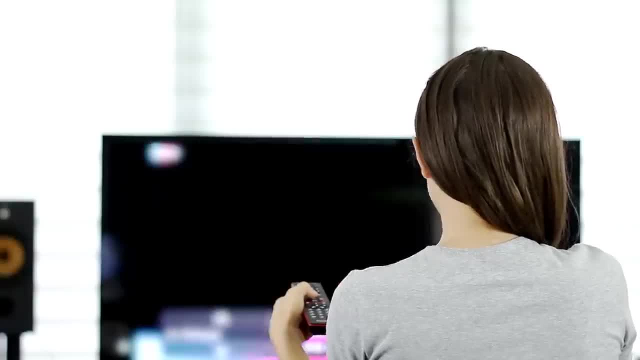 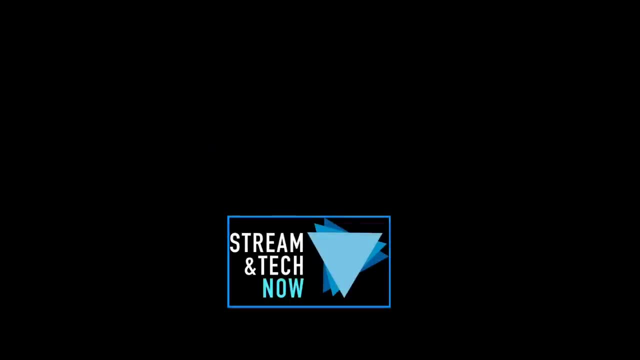 surprise. they came in at number 11, but in my opinion they should be sitting at number 12.. So that's it for me today. Let us know in the comments what is your go-to and what brand have you had negative experiences with. I'm very curious to hear what you think. 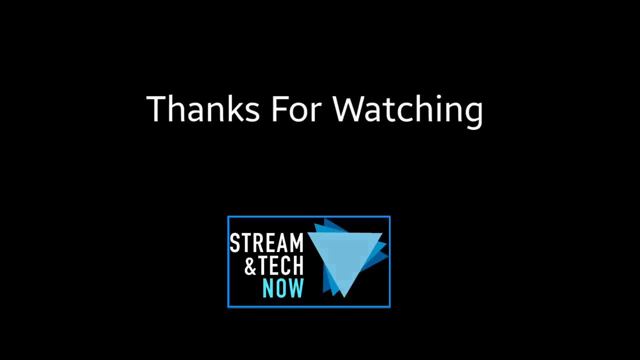 Thanks for joining and don't forget to hit that thumbs up, comment and subscribe. We'll see you next time on Streaming Tech Now.